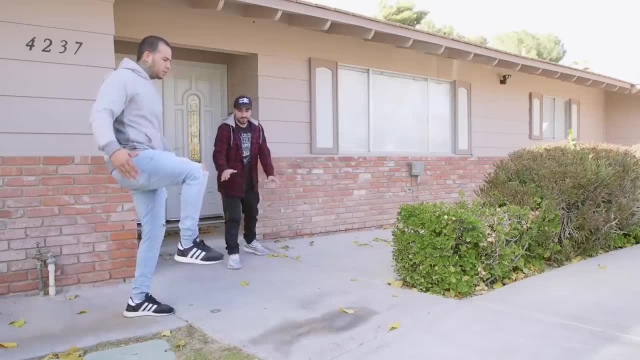 Okay, Yeah, don't push forward, Push up. Alright, so forward, move back, push up, don't push forward. Yeah, go ahead. Don't mess the box up Here. we go, Go ahead. My box is right here. 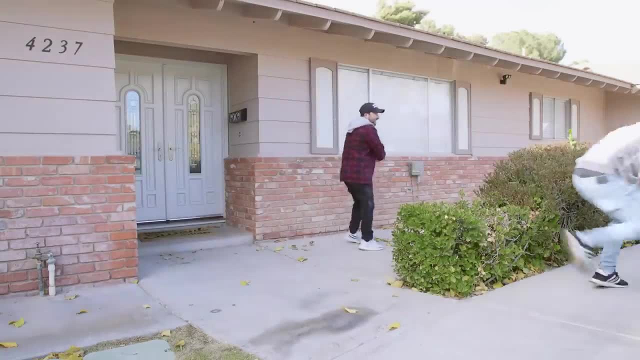 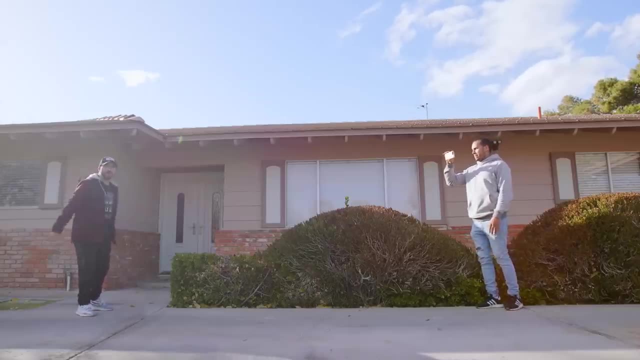 Go Yeah, three, two, one, Ah. No, There's no box. Alright, guys, Derek's doing me. I'm about to do the triple invisible box jump. You ain't never seen nothing like this, but it's so easy once you get it right. 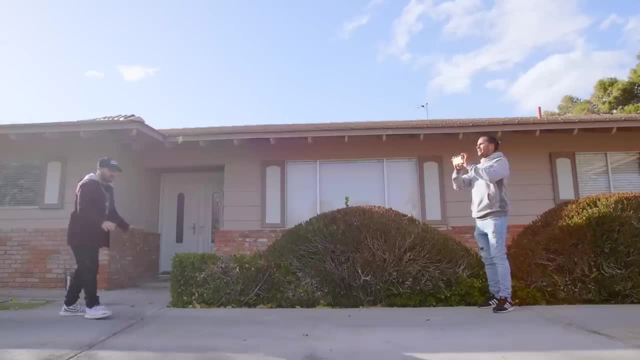 Okay, All you gotta do? All you gotta do is focus and keep your legs stiff. Watch this Ready. Hey, say what's up to Instagram Live, bro. Yo Instagram Live. check out the invisible box. jump right now, Let's go. 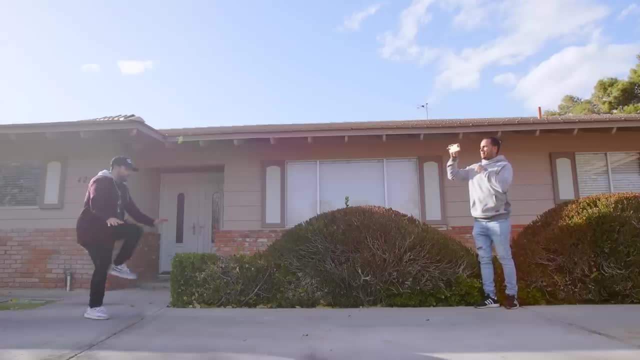 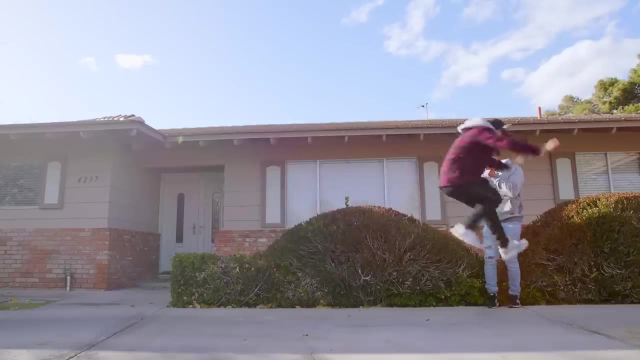 I'm measuring them. They're good to go Check me out Ready. Yeah, Don't fall, bro, You're live. Oh my God, Oh my God, Oh, What is going on? Oh my God. 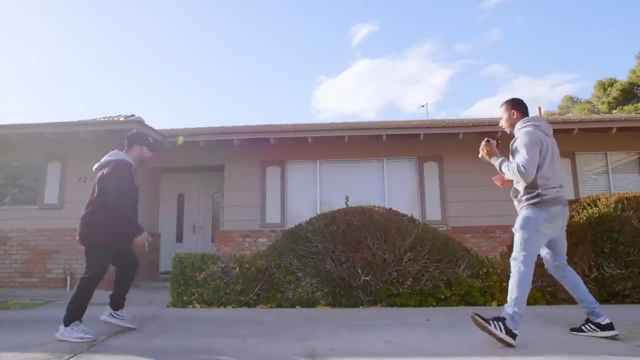 Instagram Live. there's no way, baby, Let's try it. There's no, I'm gonna try it. Let's go. Let's go, Come on. Yeah, let's do this one. I'm going here Go. 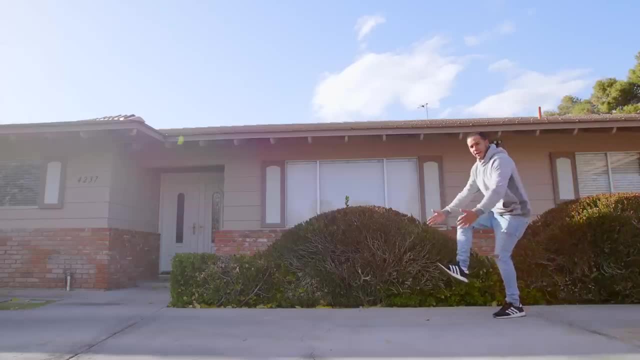 Here we go, guys. Get the legs stiff, though, All right, Legs stiff, Yeah, Here we go, Double Go. Oh, there we go. Yeah, I can't do it. I can't do it, Hey guys. 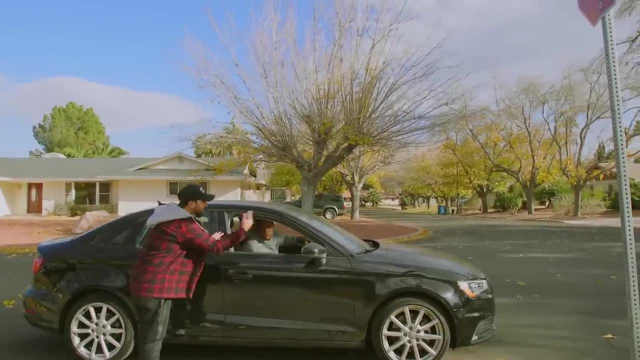 Just for the record, I think this is a very bad idea, Bro. just go. Bad idea bro. Go, Come on, Set it up Right there. Come straight at me with the car. Remember, go at least 70 miles an hour. 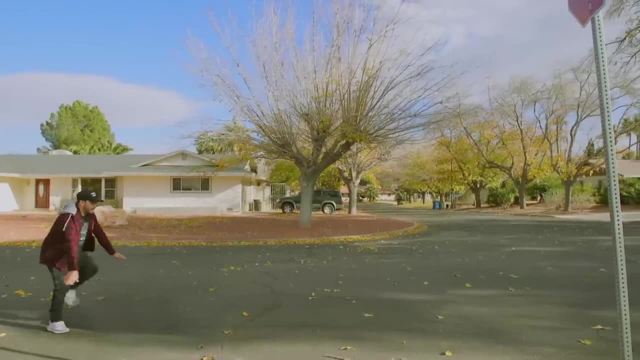 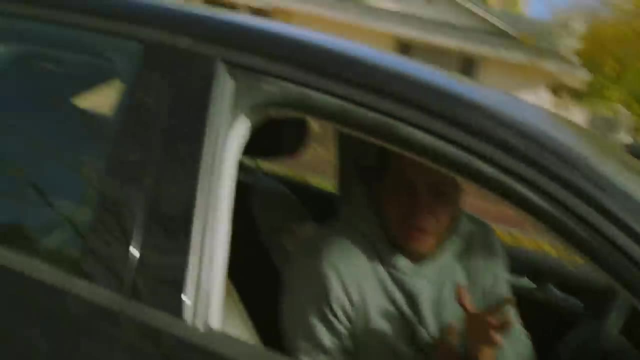 Trust me, Come on, Ready, Go Whoa. Oh, Oh my God. Oh my God Bro, that was gonna kill you. Oh my God bro, I am gonna be walking over this pool with the Invisible Box Challenge at the same time. 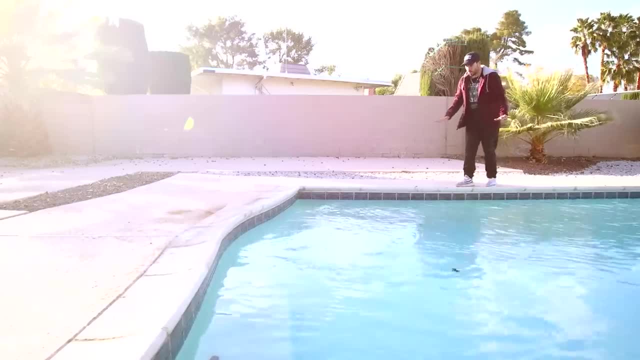 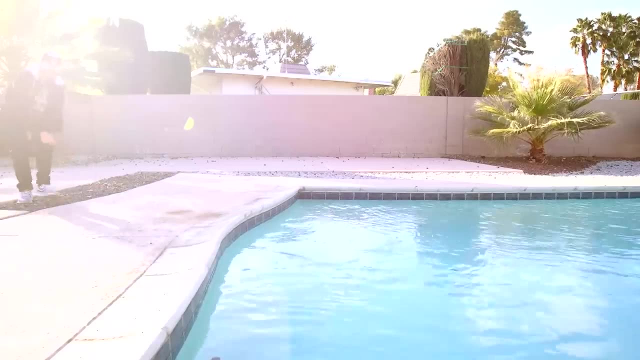